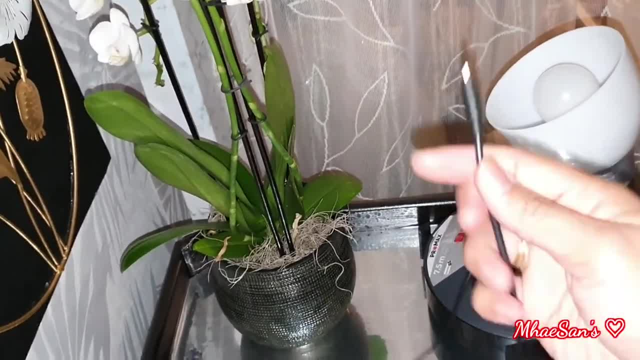 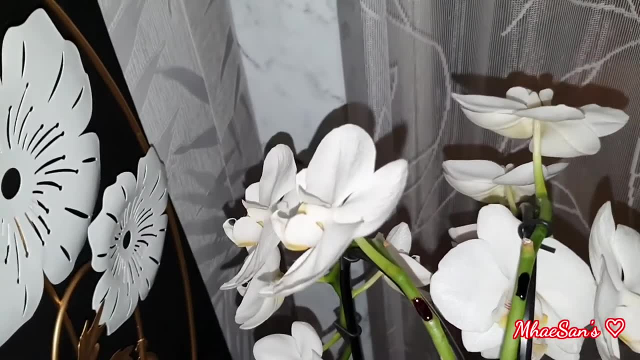 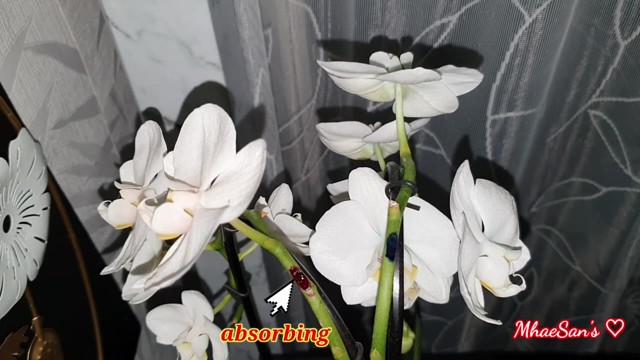 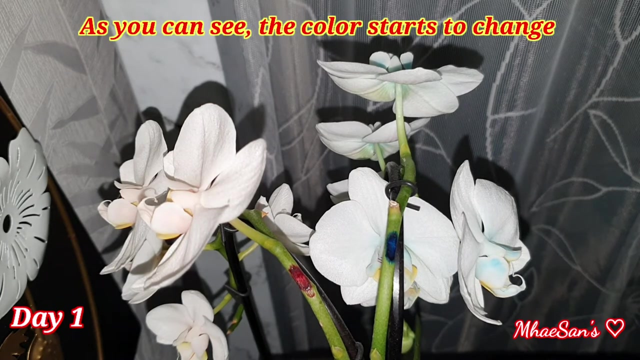 On top of my cabinet. I put the extension wire here so I will keep it charged, And the flash on the camera so it gives light even at night. I will just put it here and let it record. Okay, And there it is. 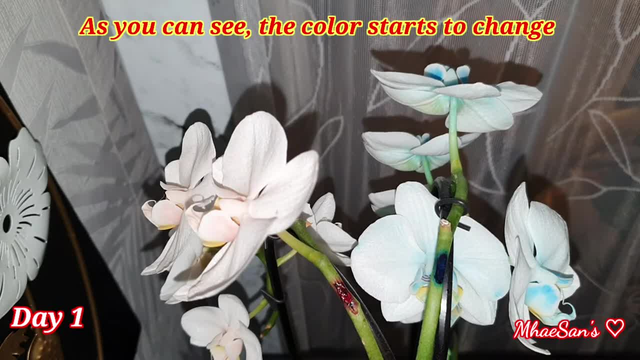 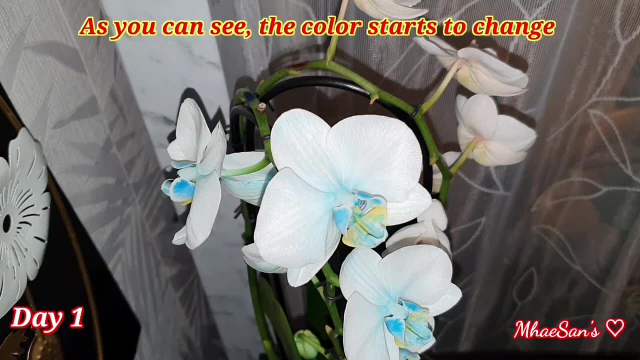 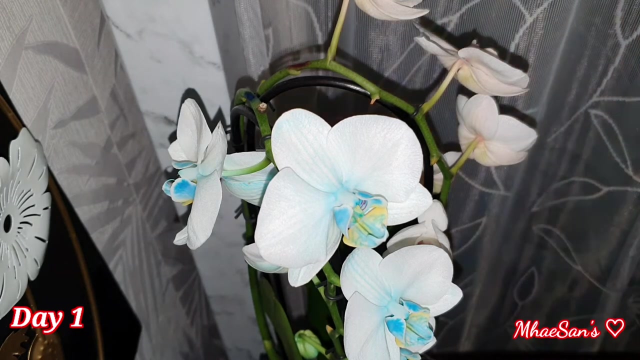 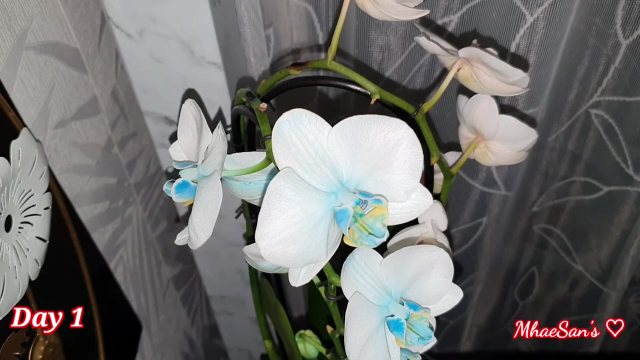 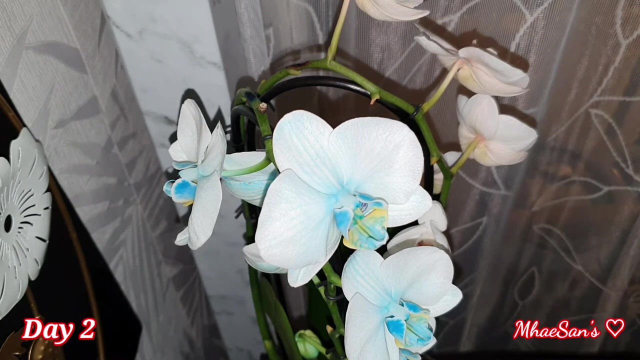 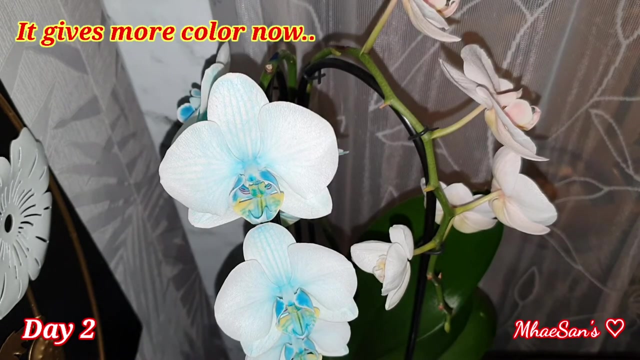 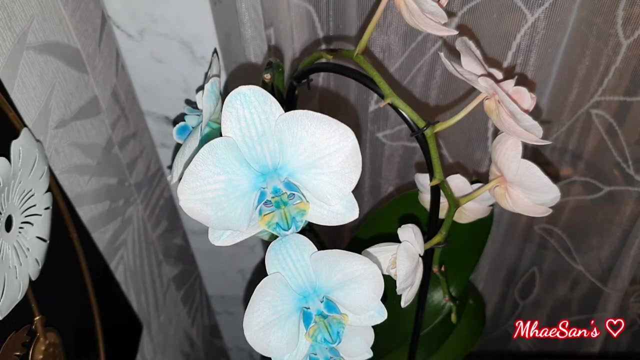 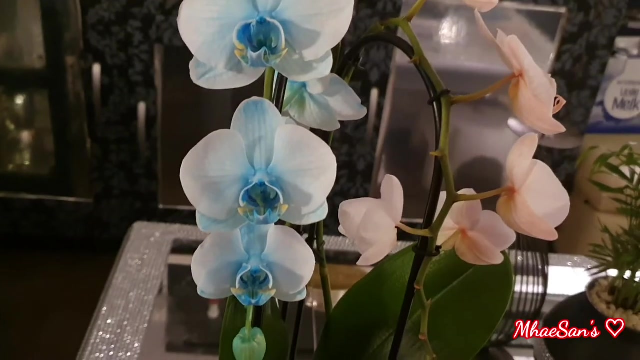 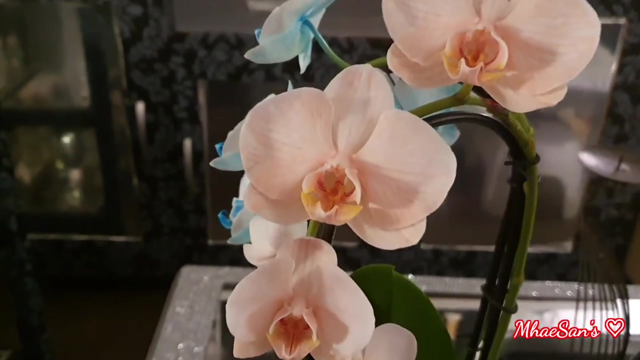 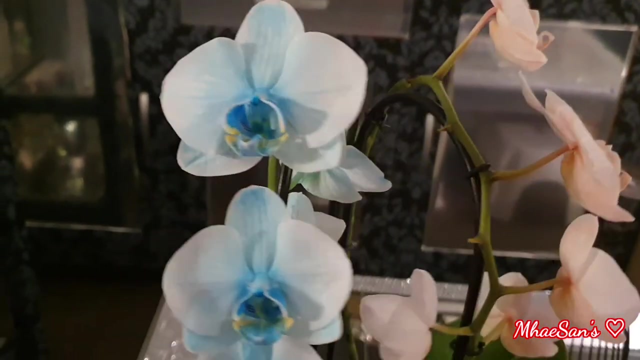 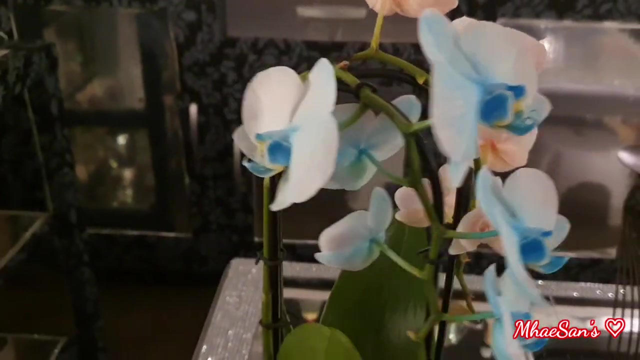